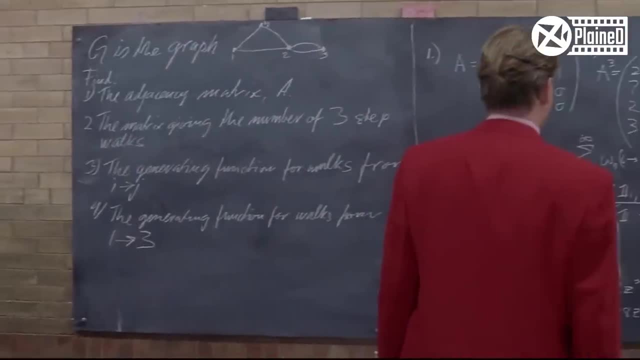 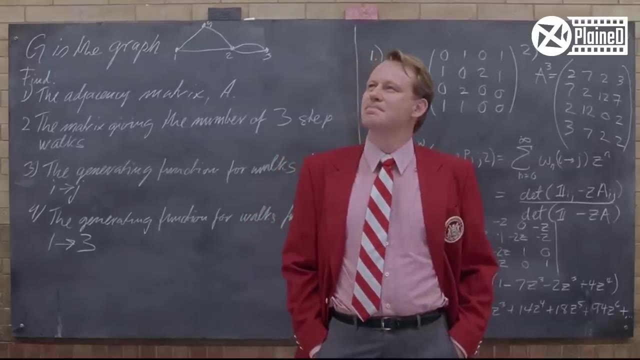 He immediately goes to check and see that someone had really solved his question. He asks some of the students if they're the ones who solved it, but he's left confused. when none of his students confirm who actually solved the question, His next class gets packed. 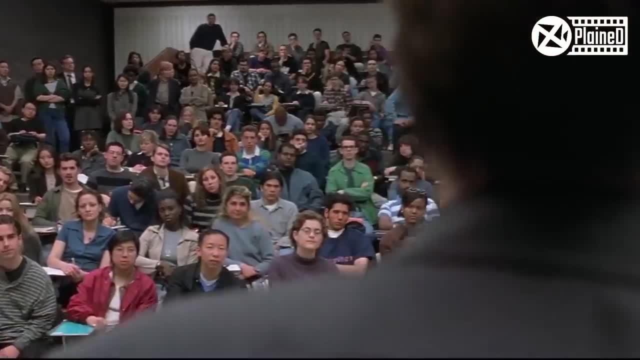 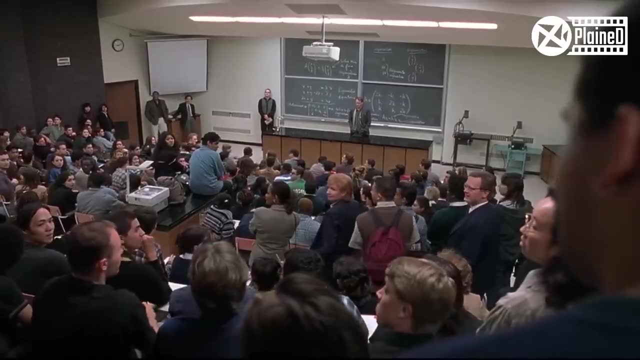 as everyone wants to know who the mysterious math genius really is, Professor Gerald calls for the person to come forward and claim their prize, but the whole class is left staring at each other, waiting for someone to step forward, With no one claiming that they solved his question. Professor Gerald tells his students that he has 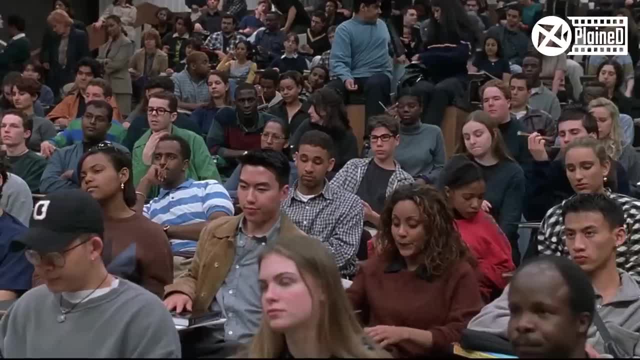 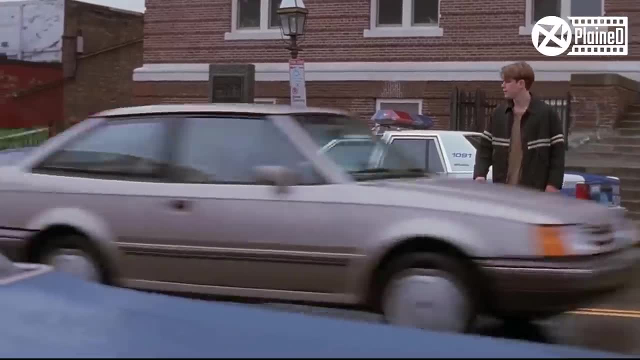 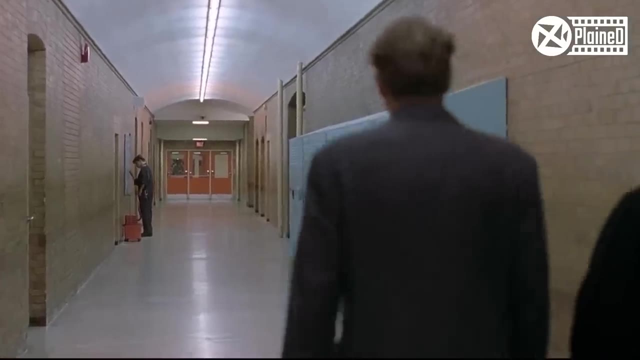 written another question, and that's it. He's left alone waiting for someone to step forward. Will, on the other hand, gets out of jail and almost immediately gets to solving the problem. At the same time, Professor Gerald comes out of his office and sees Will writing on the board. 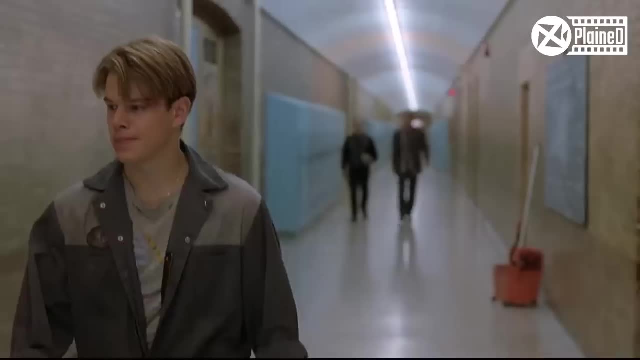 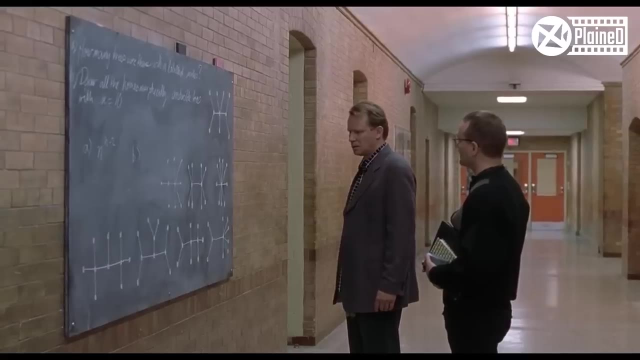 He tries to confront Will, thinking that he's just graffitiing on the board Seeing him come towards him, Will flees the scene. It's only later when Professor Gerald walks back and sees that Will had actually solved the problem, which took him two years. 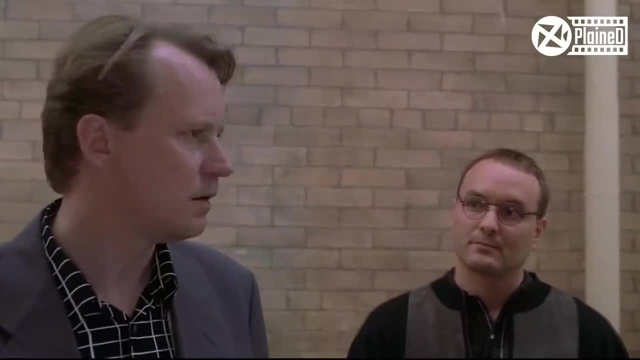 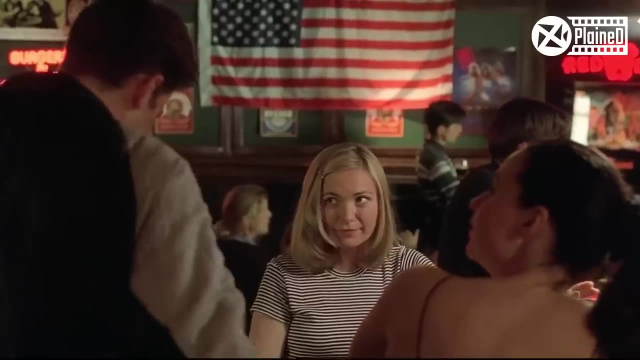 to do so. He now knows who the mysterious math genius really is. After work, Will meets his friends and goes back to a bar to get some drinks. Seeing a couple of beautiful ladies, Chucky goes up to them and starts flirting To impress the girls. Chucky lies that he goes to the same class with them. 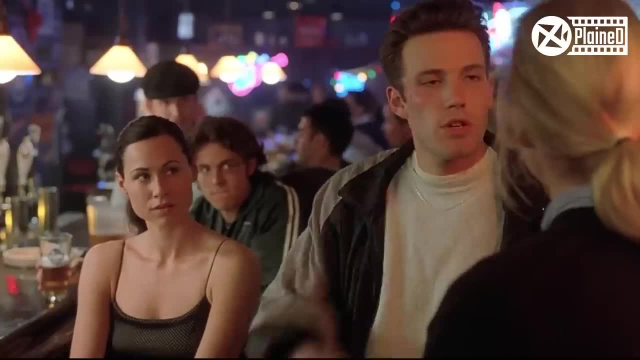 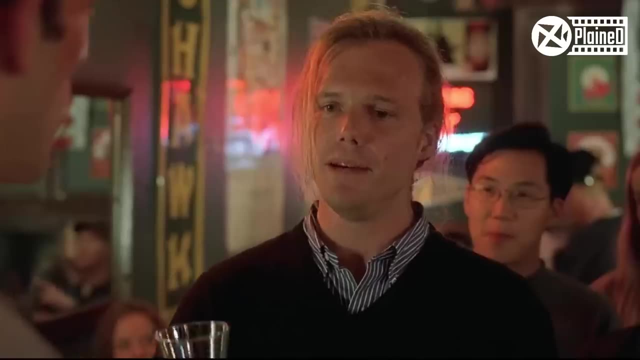 Just then a man interrupts him and asks what class he actually means, to which Chucky replies history. The man goes to the same class as those girls, so he knows Chucky is lying. He tries to embarrass Chucky by asking him his thoughts on historical. 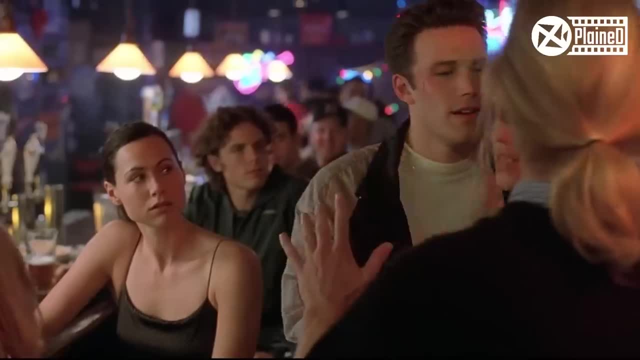 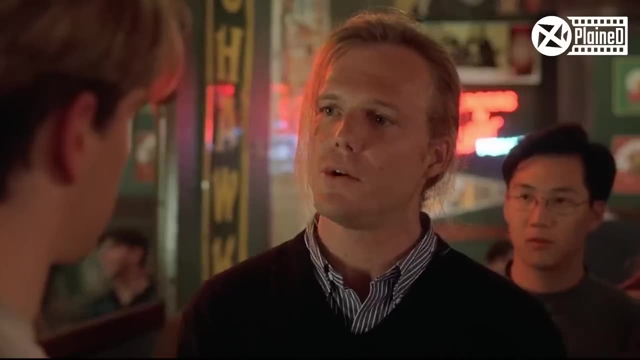 matters, Not being a history student. Chucky stays silent. so Will steps in for his friend and starts his debate with the man by laying out facts and his own thoughts. The man counters with something, but Will cuts him off and completes his entire sentence before calling him out for 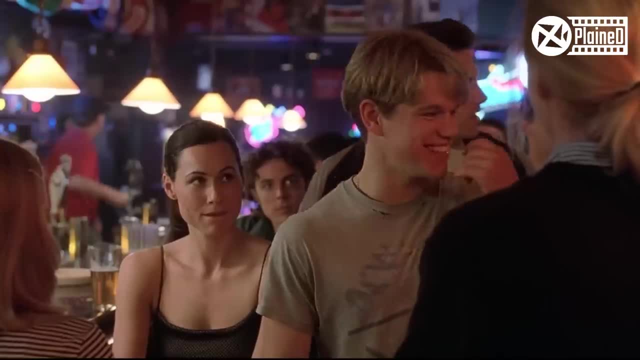 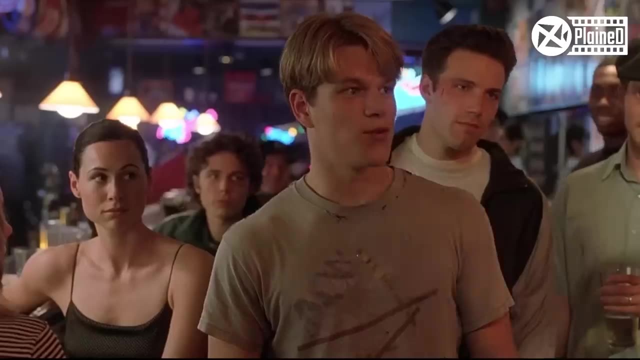 reciting a passage word by word from a book. Will makes fun of that guy for spending thousands of dollars on education which he got for free in a public library. After getting embarrassed by Will, the man walks off from there. Later, one of the girls named Skylar comes to Will and gives him her. 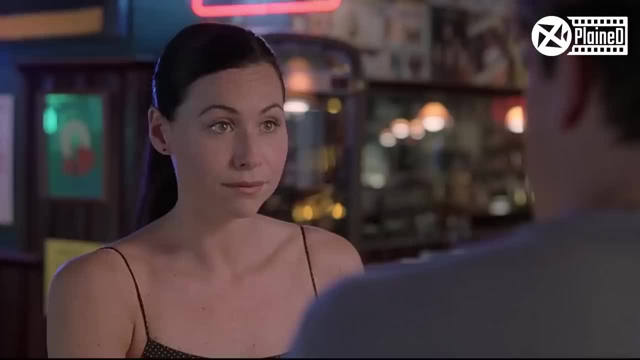 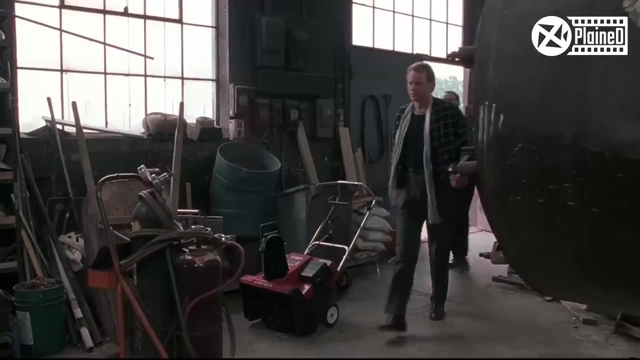 phone number. Impressed by Will's earlier show of intelligence, Skylar asks him to call her so they can go out for drinks in the future. Will later shows off that number to the guy who was trying to act smart. Meanwhile, Professor Gerald has been searching for the janitor who solved his complex. 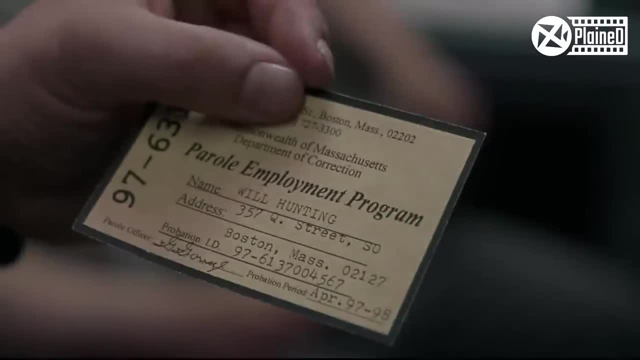 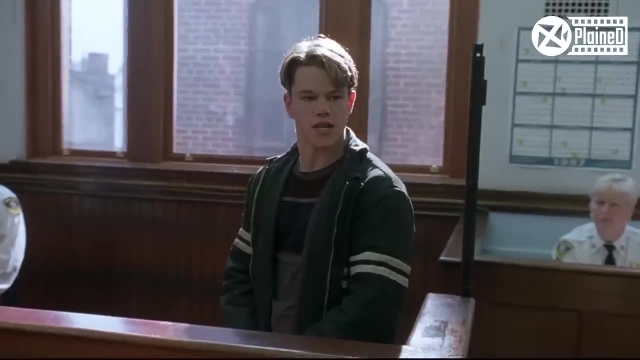 mathematics problem. After asking a few people he finally gets contact information on Will. He shows up at the court hearing of Will in the case of him assaulting a police officer. Will defends himself in the case, but the judge tells him that he has a lot of prior cases of petty 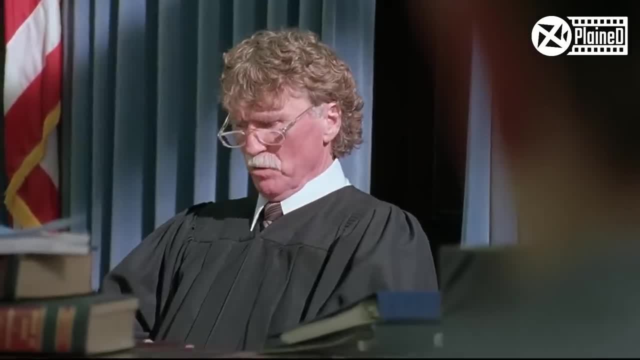 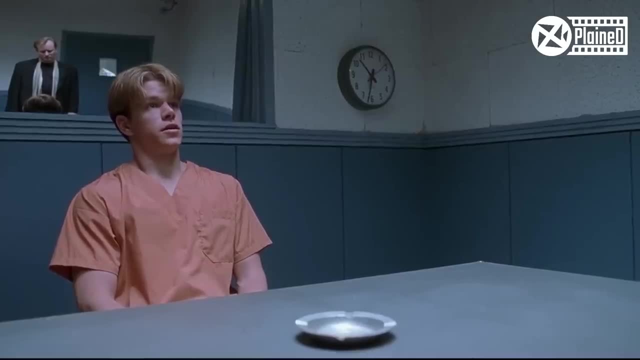 theft and assaults. Will then asks the man to give him the phone number. Will then asks the man to call the police. The judge says that he can't turn a blind eye on everything that Will has done and gives him jail time with bail of $50,000.. With that Will gets sent to prison. but there he meets. 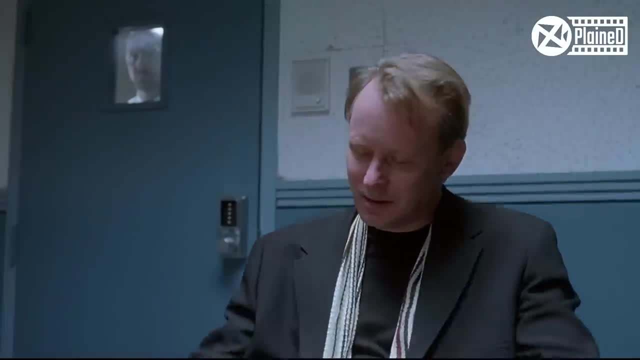 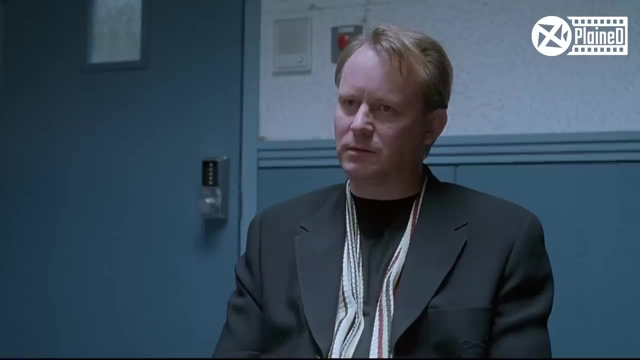 Professor Gerald, who has a proposition for him. He tells Will that he has spoken with the judge and is ready to pardon him. but Will must agree on two things. The first condition is that Will takes mathematics class with Professor Gerald, and the second condition is that he must get. 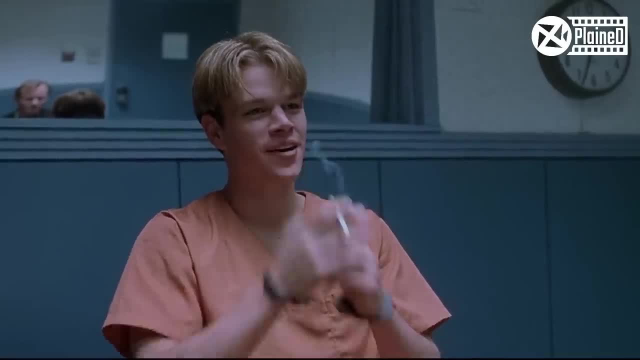 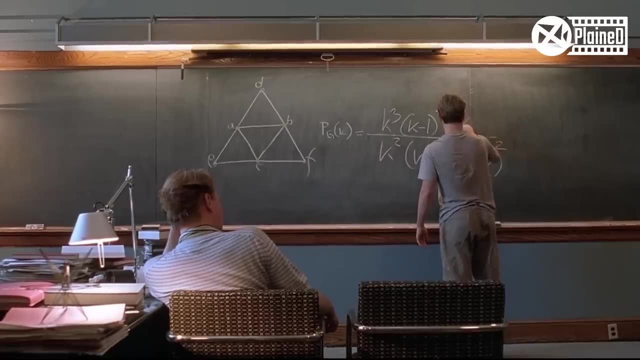 counseling. Will laughs at that suggestion of him seeing a therapist. but to avoid jail time he has no option but to agree to all the conditions laid out before him. Soon he starts to take mathematics class with Professor Gerald, who is amazed and proud of Will's. 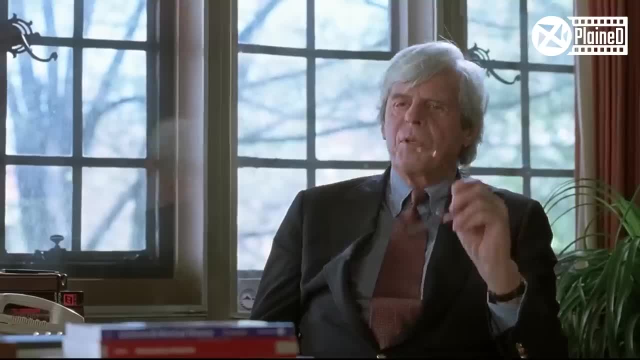 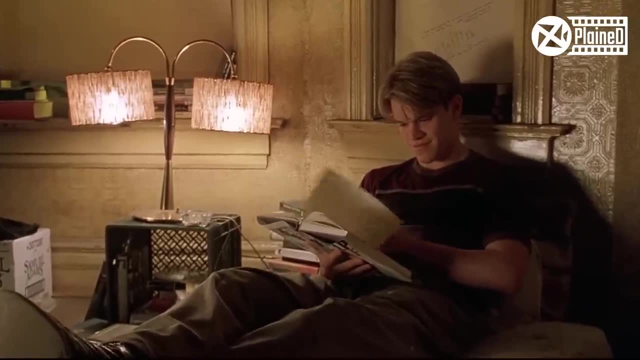 intelligence. Next, he has to get counseling from a therapist, but despite how many of them he visits, Will refuses to open up and even makes fun of them. He reads their books the previous night and makes a mockery out of them during his counseling. As a last resort, Professor Gerald, 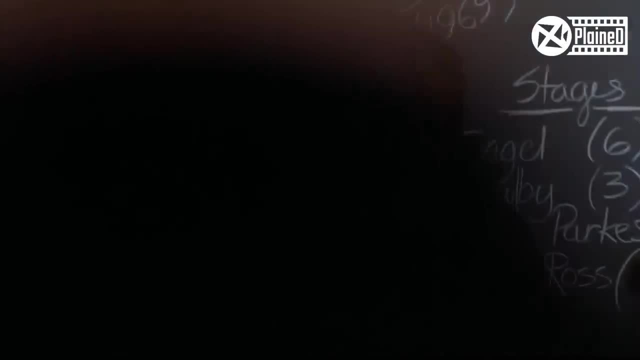 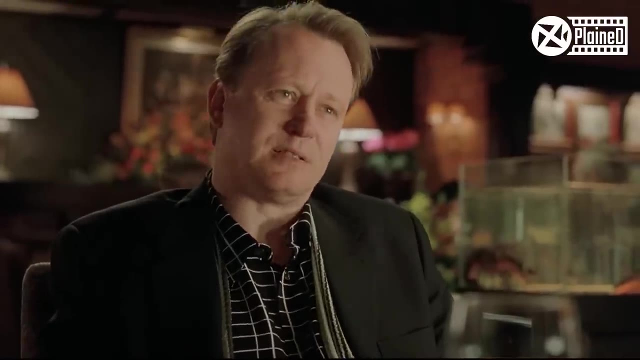 turns to his old friend Sean McGuire for help, who now teaches psychology at a community college. Sean at first says that he doesn't have time to do this, but Professor Gerald insists he should help Will, saying that he's a genius and his counseling can help Will achieve the best in 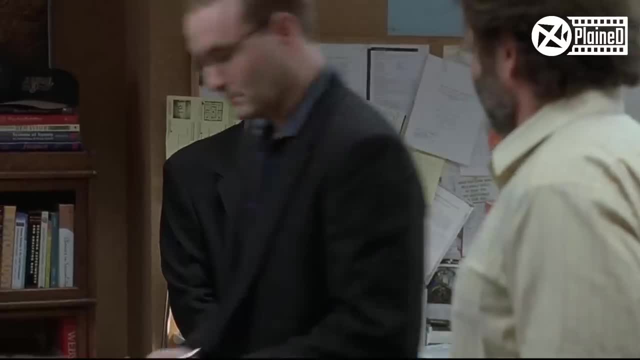 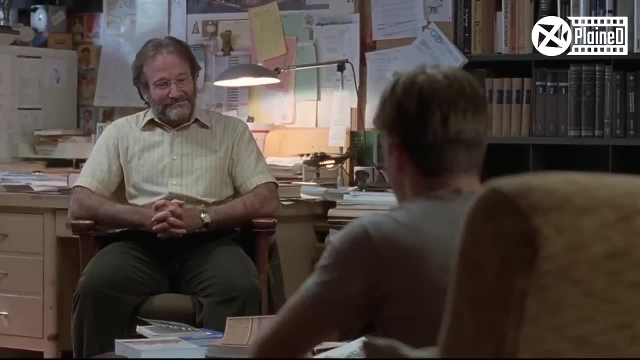 his life. Sean finally agrees and meets with Will In his first therapy session. Sean asks Professor Gerald and his assistant to leave the room. Just like with his previous therapist, Will begins to make fun of Sean's book collection. Sean knows that it's Will's defense mechanism and that he's deliberately trying to make him mad. 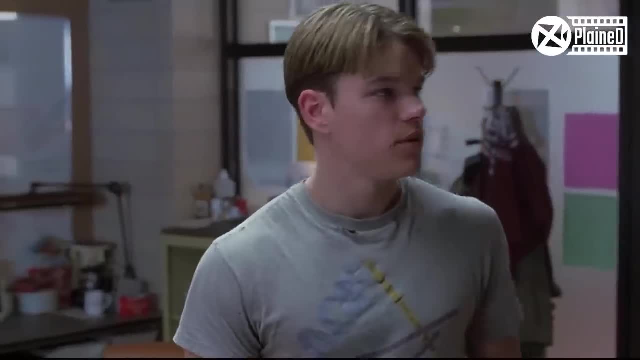 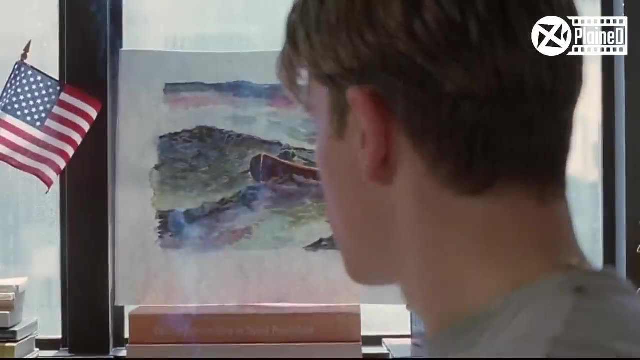 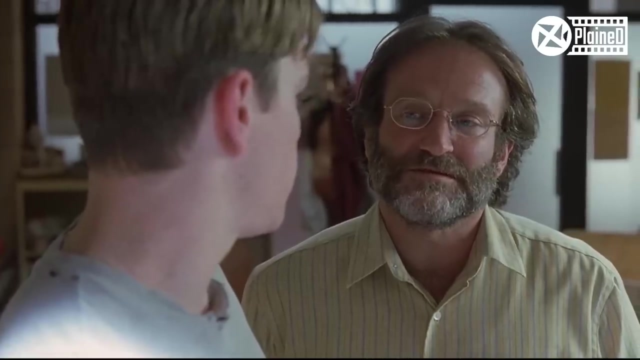 so Sean keeps his composure and engages in normal conversations. Will then notices a painting that was painted by Sean himself. Looking at the painting and quoting several art books, Will makes several false assumptions about Sean's life. Sean, yet again, doesn't react to Will's insults, but when Will brings up his wife in the conversation, 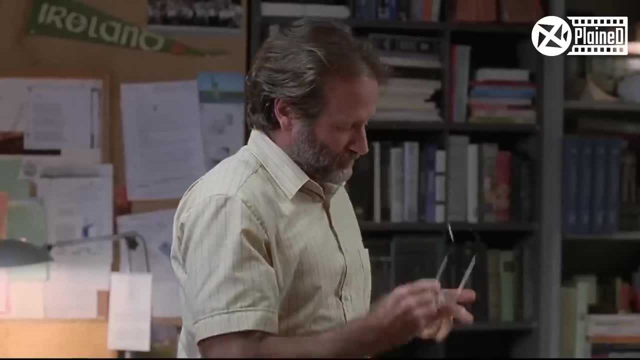 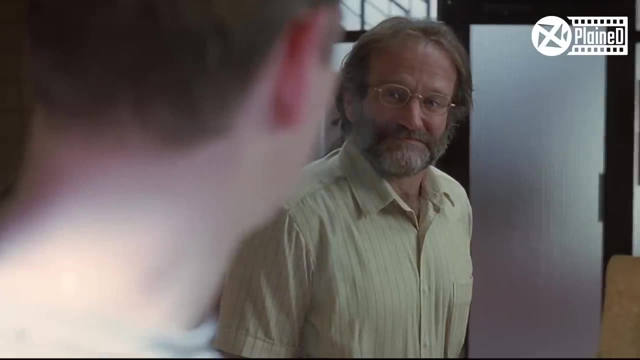 Sean gets a little bit irritated. Will realizes that Sean's weak point is his wife, so he keeps bringing her up. He asks if Sean's wife was cheating on him. Sean completely loses his mind and grabs Will by his throat. Will then says that Sean's wife was cheating on him and he 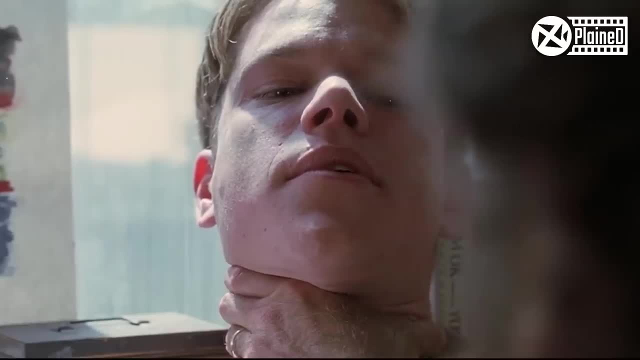 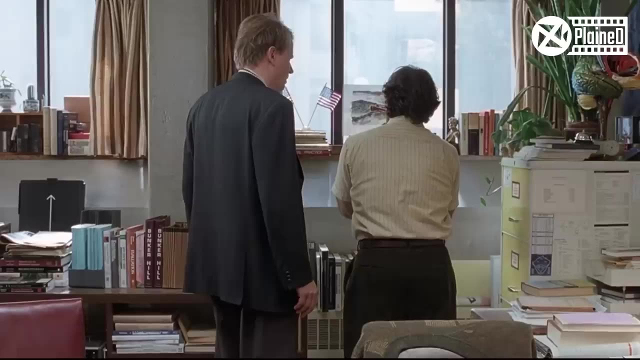 warns Will to never disrespect his wife. Just then Will tells Sean that the session is over. Sean lets go of him and Will goes out, believing he yet again managed to break a therapist. Seeing Sean's mood, Professor Gerald believes he won't agree to do more sessions with Will. 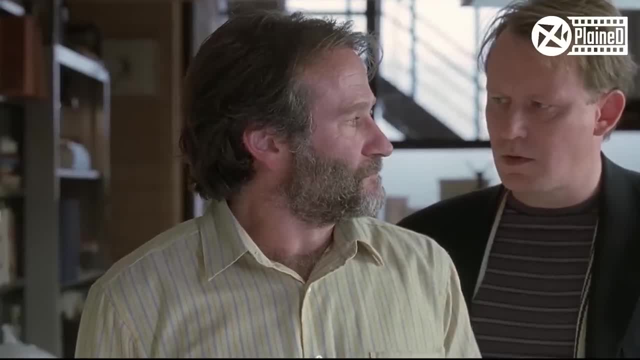 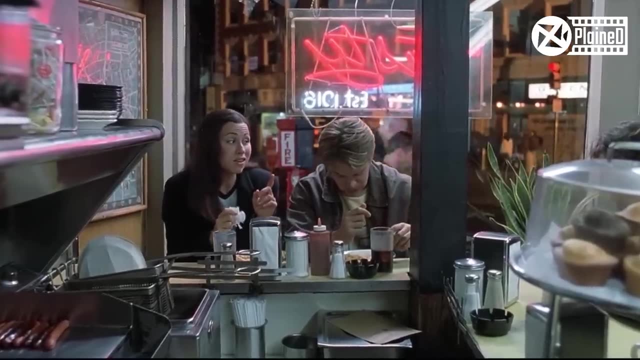 But surprisingly Sean asks to continue his sessions with Will from next week After his counseling Will goes out on a date with Skyler. On their date, Will finds out that Skyler comes from a very rich family and is studying at Harvard. The two immediately get along and 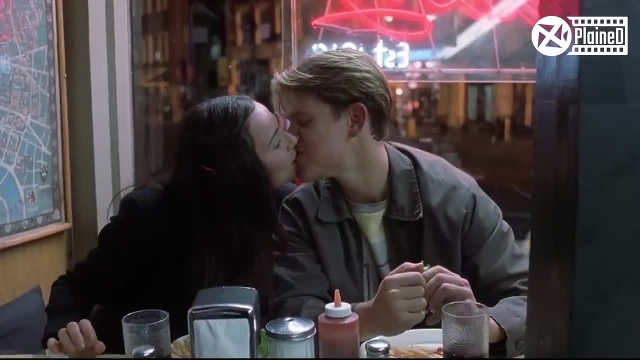 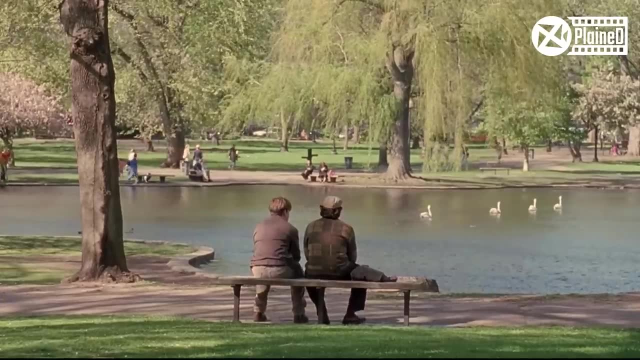 enjoy their time with each other. To end the night of their first date they even share a kiss. Will shows up next week at Sean's office who tells him to come outside with him. Sean takes Will out to a park and talks to him. He tells Will that he thought a lot about what. 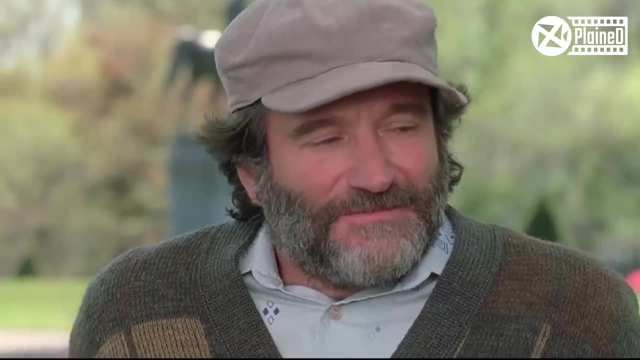 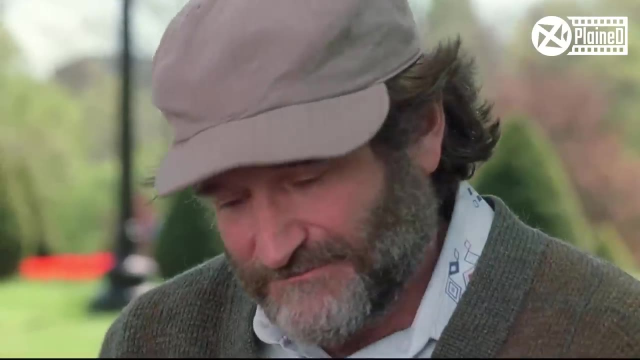 he said and about his painting, and after a while came to realize that Will's just a kid who doesn't know what he's talking about. Sean tells Will that, just like how he cannot make assumptions about someone else's life by reading a few art books, 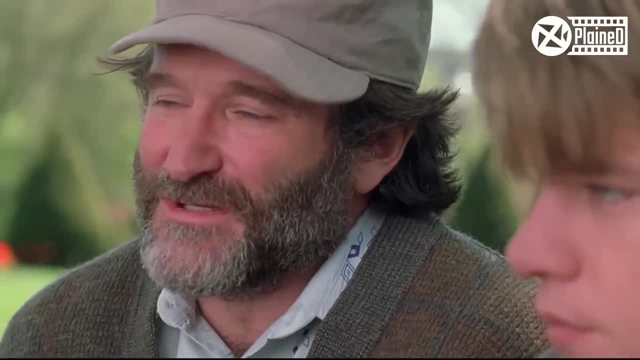 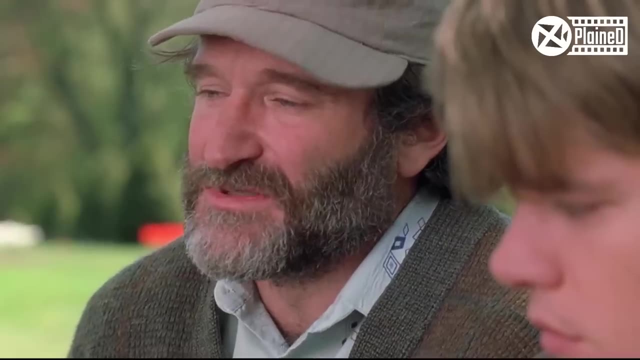 he cannot tell about Will's problems by just having a degree in psychology. Sean says he understands that Will doesn't want to speak as he's scared of what he'll say. But at some point he'll have to start talking or else he'll never experience the best things in. 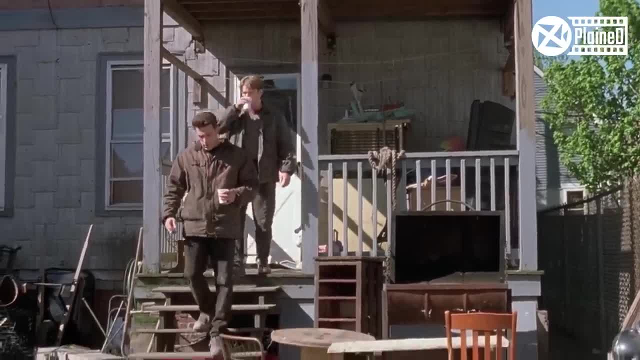 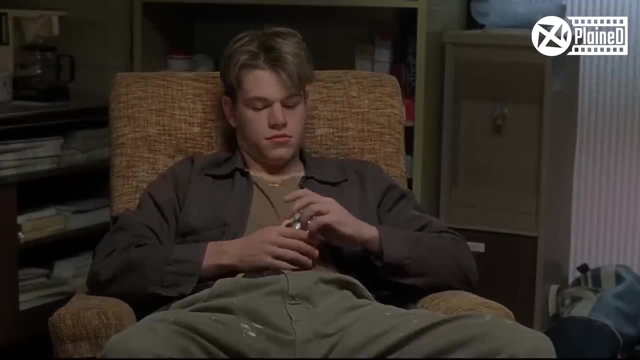 life. Will goes back to his life where his friend Chucky picks him up and drives him to their workplace at a construction site. He calls Skyler, but he's afraid of talking to her On his third therapy session with Sean. Will doesn't speak a word, and so does Sean. They just 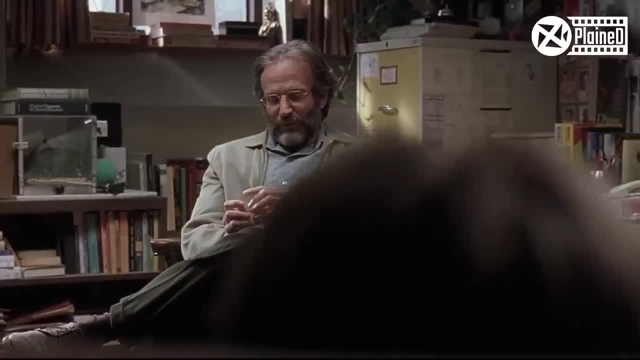 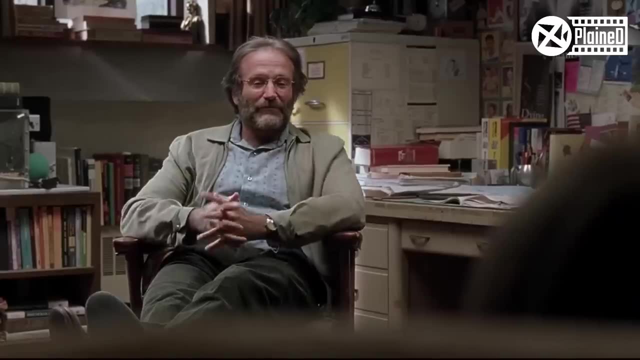 keep silent for the whole hour. The fourth session starts in similar fashion, with Will not speaking a word, but then, out of boredom, Will tells a joke to Sean, Taking it as an opportunity. Sean asks if he has a girlfriend. Will then tells him about Skyler and how he hasn't been in contact with her. 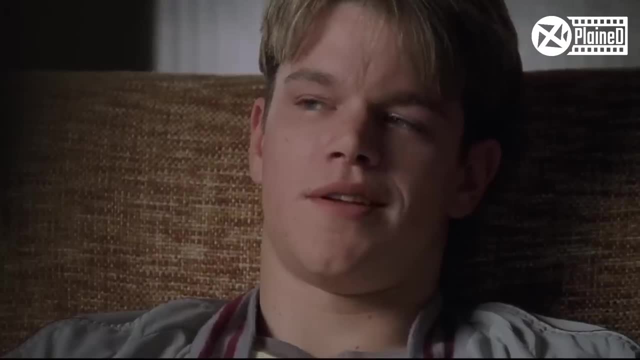 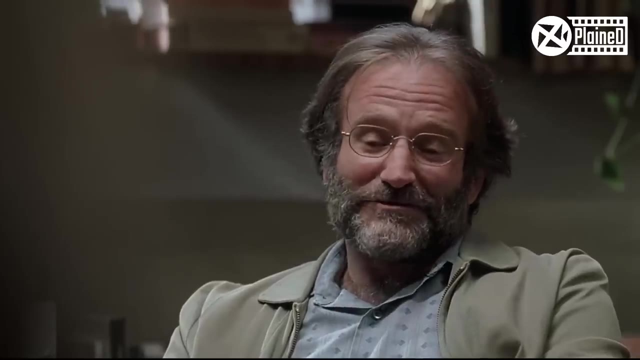 ever since their first date. Sean asks why, and Will replies that he feels Skyler is too good for him and if he continues talking to her it'll just ruin everything. Sean then tells him that no one is ever too good or perfect. Everyone has flaws. but what matters most is if that person is. 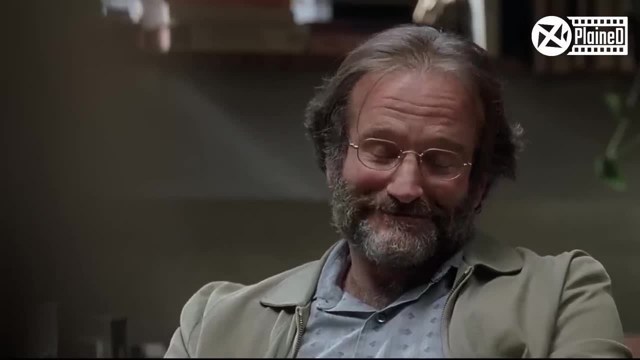 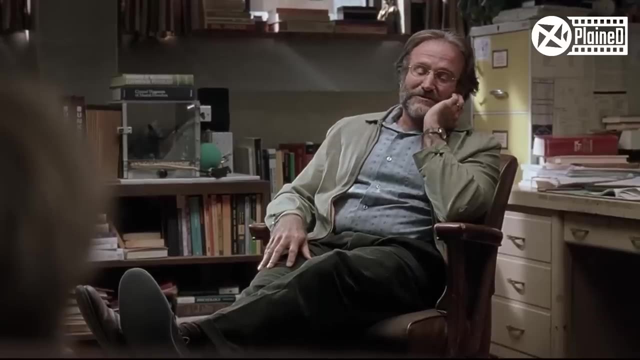 perfect for you or not. To get the message more clear to Will, Sean tells him about his wife. The most beautiful person he ever saw and the one who he fell in love with used to fart in her sleep. This changes the whole atmosphere inside the room. Will and Sean start to laugh uncontrollably. 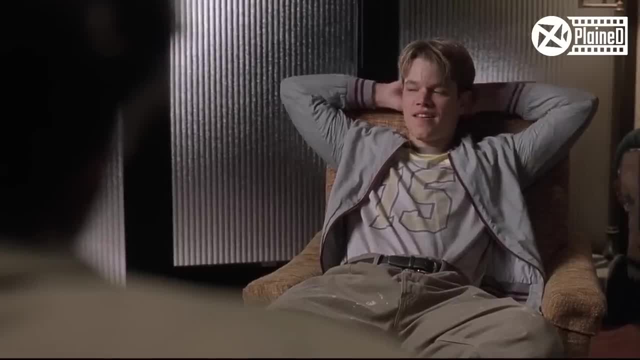 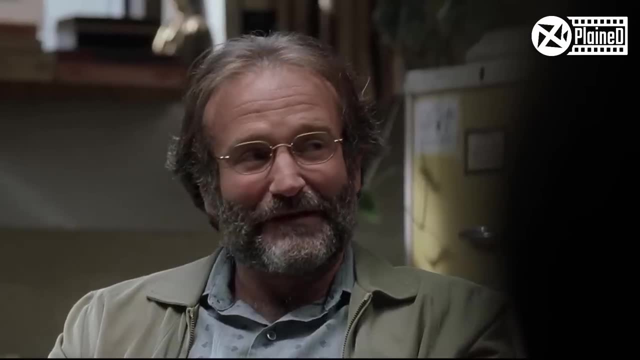 At this moment they get closer to each other and Will starts to be comfortable around Sean. The session ends with Sean advising Will not to think that Skyler's too good for him. He should rather just ask if they'll be happy together. Will is so concentrated on what Sean 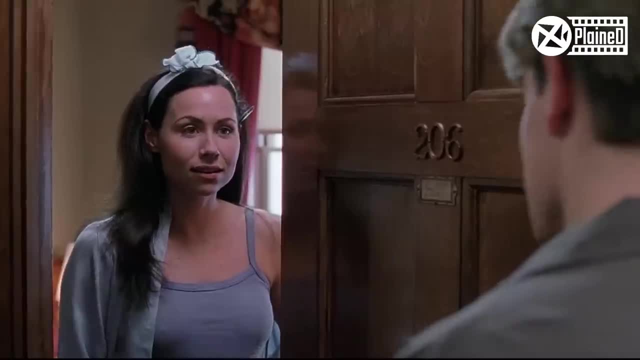 just said that he has to be reminded that their session's over. Encouraged by Sean's words, Will goes to Skyler's dorm and asks her out on a date with Skyler. Will asks Skyler if Skyler's okay after the plan and asks her out again. Skyler says that she wants to go out with him. 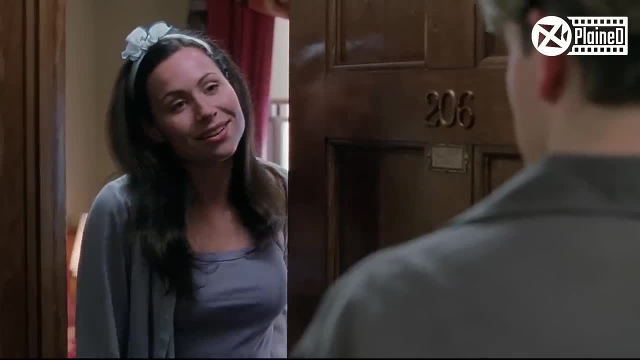 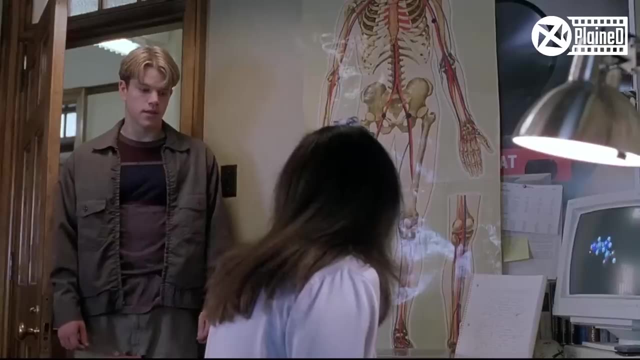 but she has a very complex problem to solve which can take her hours or even days. Will cannot wait anymore to see her, so he solves the problem on a napkin and he hands it over to her, With nothing more to worry about. Skyler and Will head out for their second date. Skyler asks. 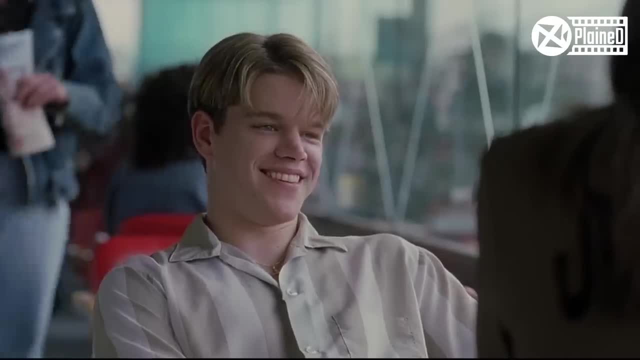 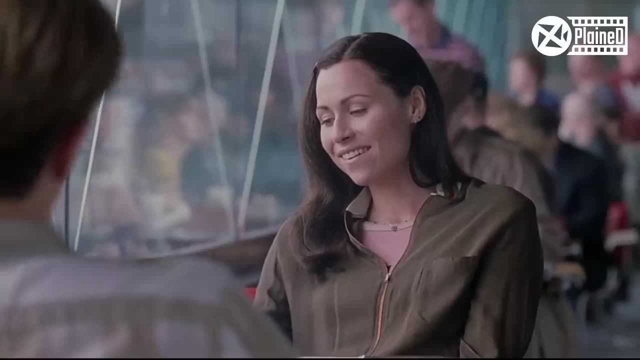 Will about his family, and Will lies to her that he has 12 brothers. Skyler asks Will to tell her the names of each of his brothers, and Will answers with 12 random names in a sequence, Doubting if Will is telling the truth. Skyler asks Will to tell the names of the brothers, and Will 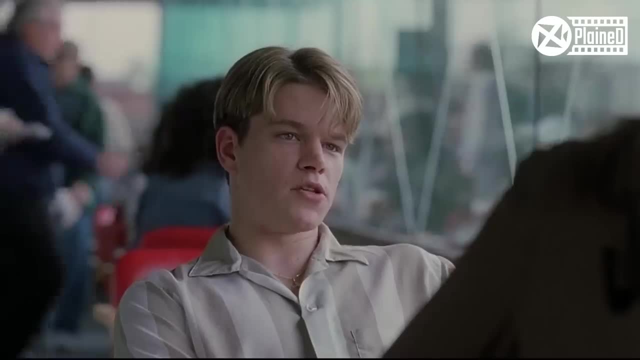 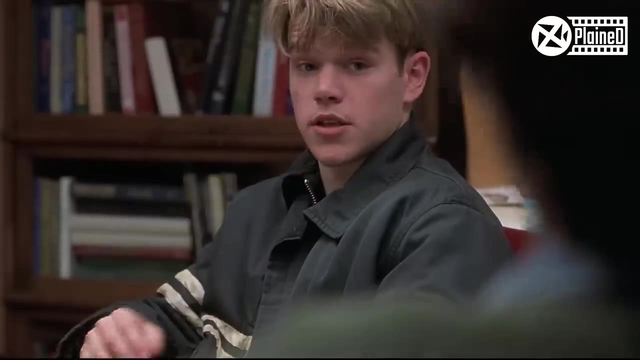 ask him to say them all again But, being the genius he is, Will repeats the name in their correct order. He meets Sean on his next therapy session and asks if he's ever regretted meeting his wife, given that after she died, he was left with a great pain to deal with. To answer his 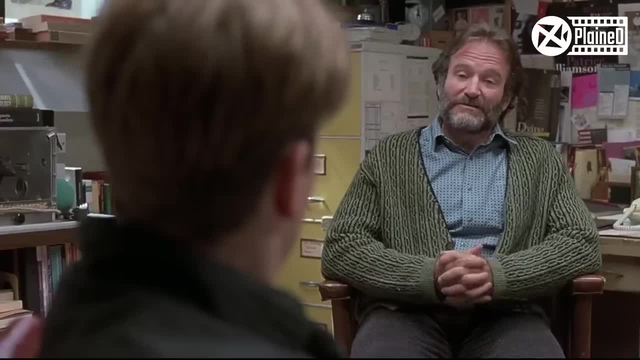 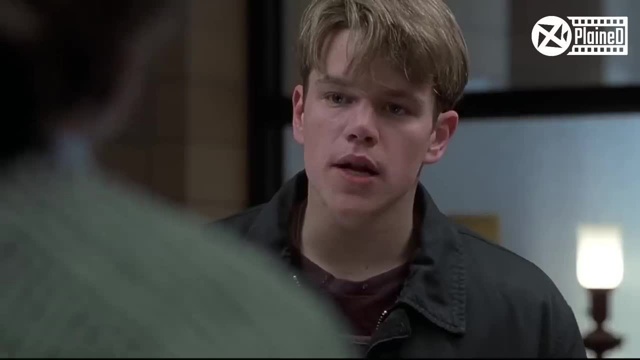 question. Sean tells him the story of how he met his wife. He says that he first saw his wife while waiting in line with his friends to get tickets for what would be an iconic baseball game. Will gets excited, thinking that Sean watched the game live in the audience and not on TV. He asks about 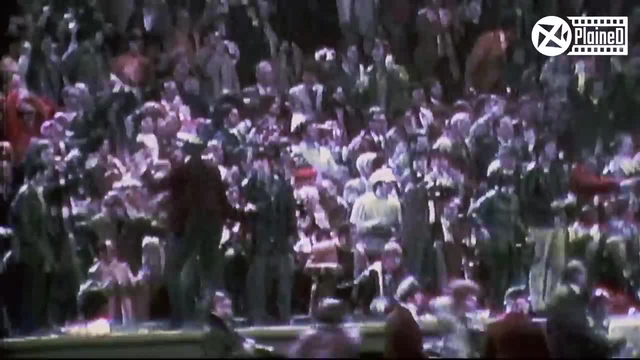 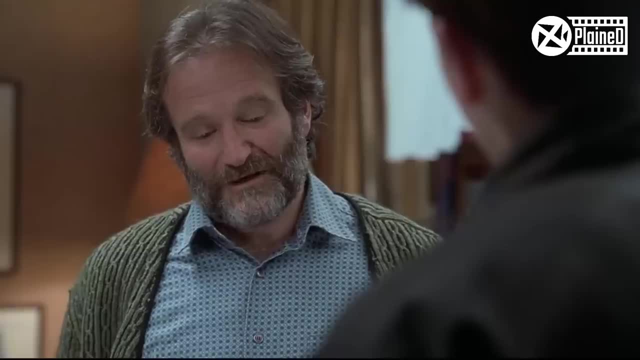 the moment and Sean details everything that went down in that game. But then Sean reveals that he just watched the game later on TV, as if he left his friends to go out on a date with the girl he just met. the girl who would turn out to be his wife Will simply cannot believe that Sean gave. 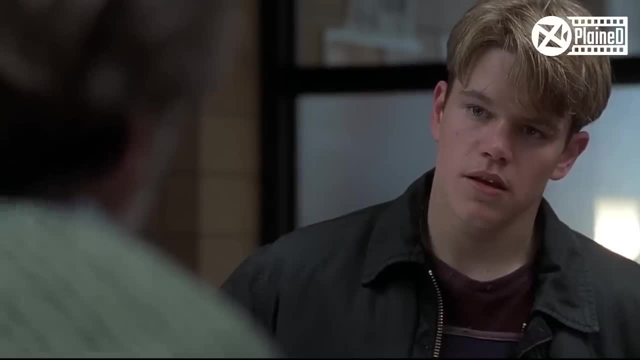 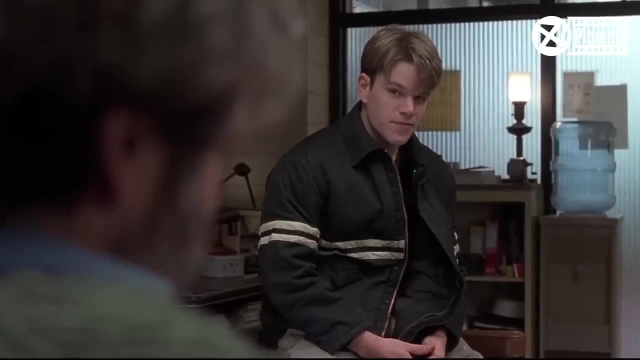 up on a historical game just so he could spend time with a girl. Now back to Will's question. Sean answers that he never regretted not watching that game live in the audience and he certainly has no regrets meeting his wife and having her in his life, even though it was only for a few years. 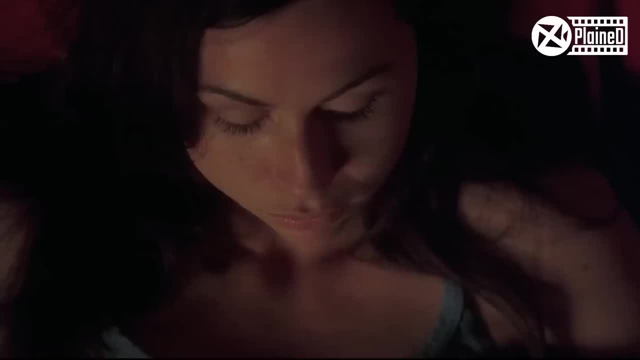 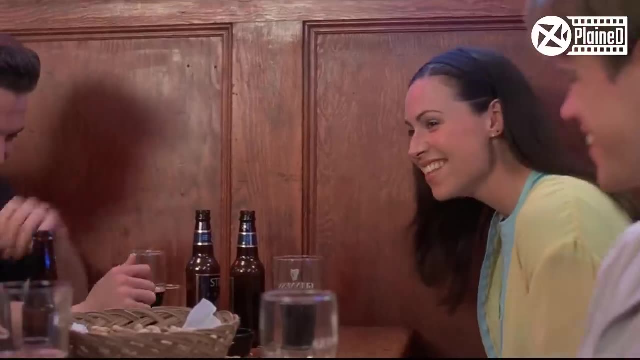 While being together, Skyler asked Will to introduce her to his friends and family. Will is still lying to her about his life, but he reluctantly agrees to introduce her to his friends. Skyler, Will and his friends meet at a bar and Skyler seems to like his friends. She enjoys her time with them. 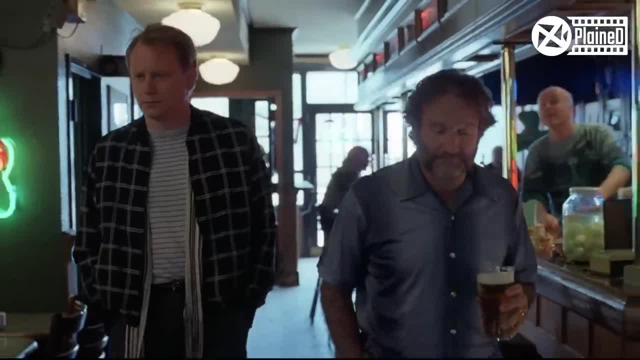 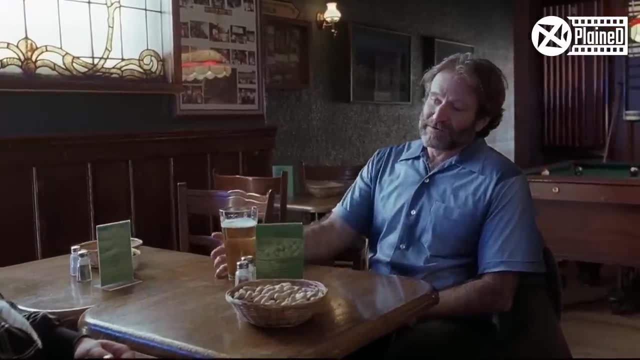 and also cracks a few jokes, which gets everyone laughing. Meanwhile, Professor Gerald asks Sean about Will's progress. Sean answers that Will has slowly began to open up, but he'll need more time before he feels completely comfortable to speak about his life and why he's afraid of trusting. 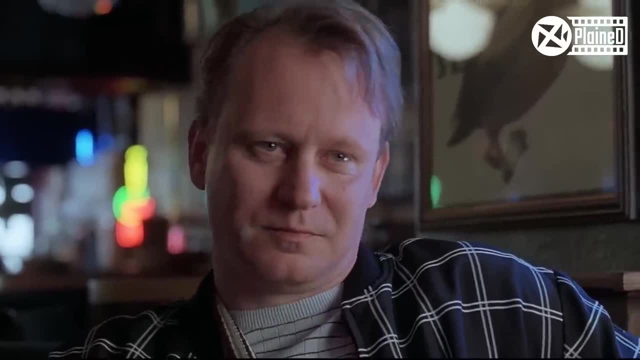 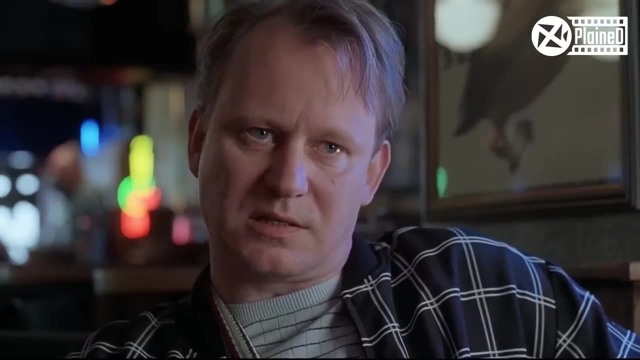 anyone. Professor Gerald reveals that he's been arranging job interviews for Will at top mathematics institutes and once his mental problems are gone, there won't be anything stopping him from making his name in the mathematics field. Sean protests that they shouldn't be the ones making. 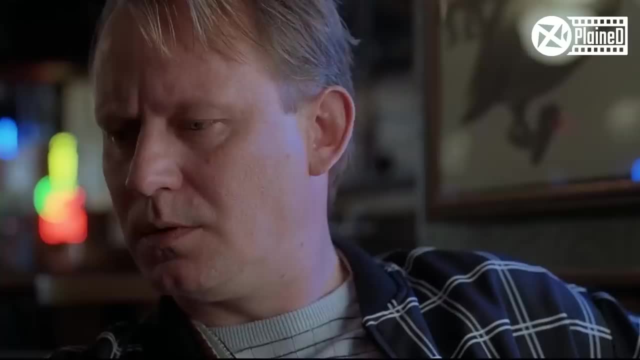 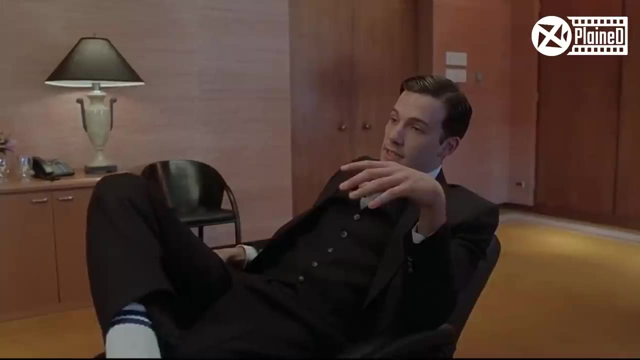 life decisions for Will and should support him on what he wants to do. But Professor Gerald is adamant that he won't let Will's talent go to waste. However, Will doesn't want to get a job like that, so he sends his friend Chucky to the interview in place of himself One night, while 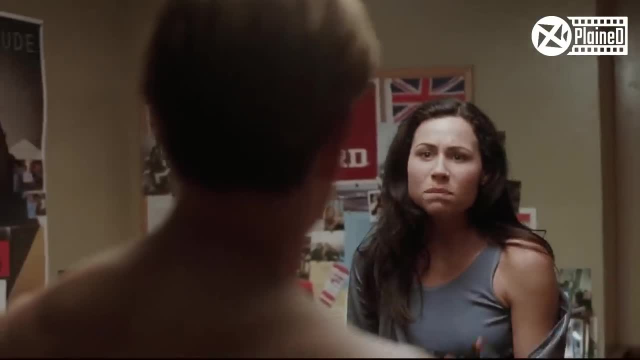 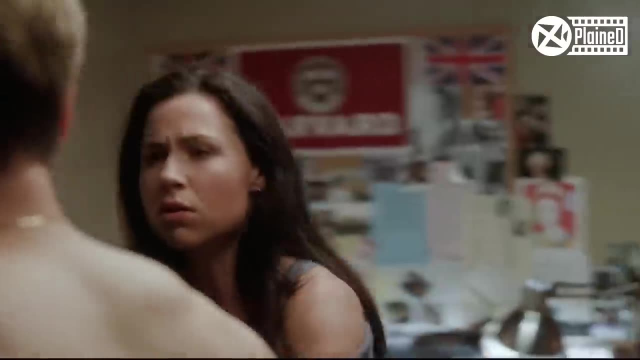 talking about their lives. Skyler asks Will to move to California and Will says he's going to California with her. Hearing what Skyler wants, Will starts to panic and says that he can't move out with her. Skyler asks why he's afraid of committing to her and why he never tells her the truth. She 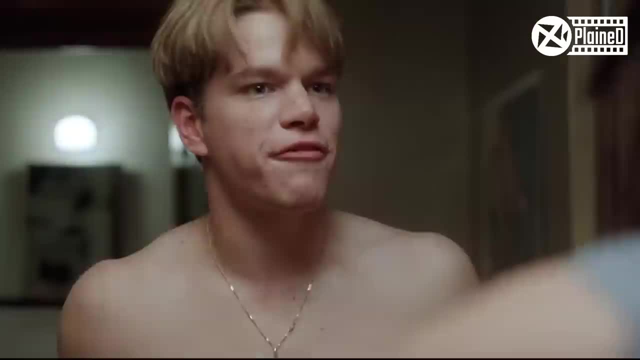 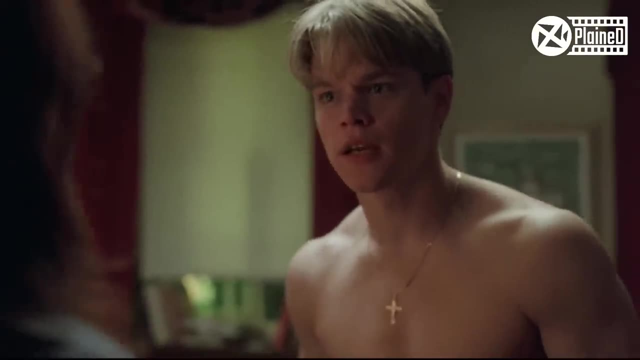 brings up how Will lied to her about having 12 brothers. After being called a liar, Will completely loses his cool. He tells her that he was an orphan and spent most of his life moving from one foster parent to another. He further tells her how he was abused and beaten by his foster father, Skyler. 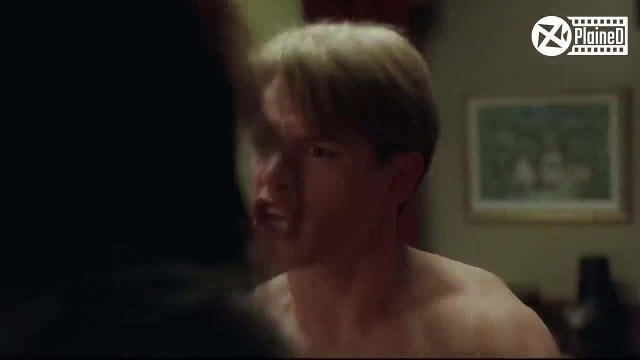 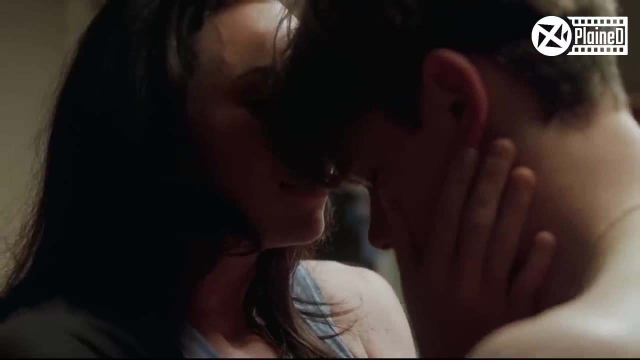 starts to cry and tells Will that she wants to be with him and help him, But Will pushes her away, saying he doesn't need anyone's help. It gets clear that Will has a fear of abandonment, where he believes that anyone he loves will walk away from his life. Skyler cries. 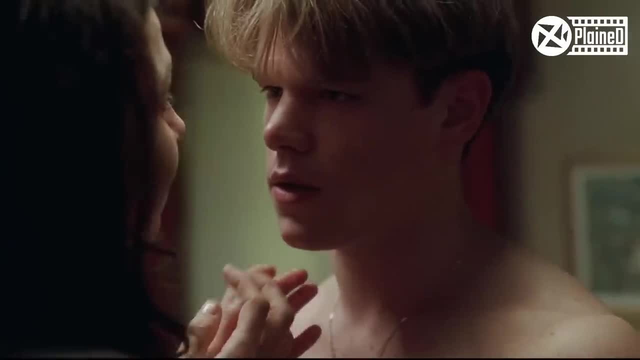 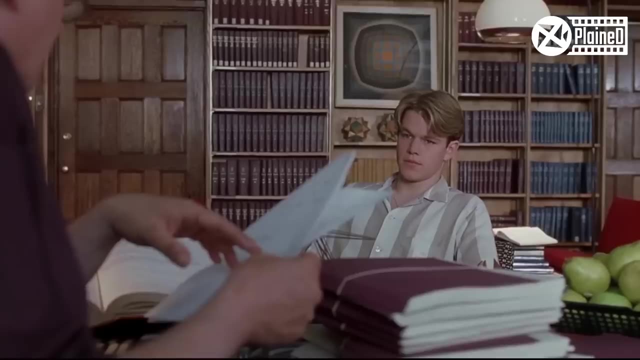 that she really loves him and will not leave him. But Will lies that he doesn't love her back and gets out, leaving Skyler to cry alone in her room. After Professor Gerald's persuasion, Will agrees to go to a job interview. Will shows up at the interview but makes no attempt to get hired. 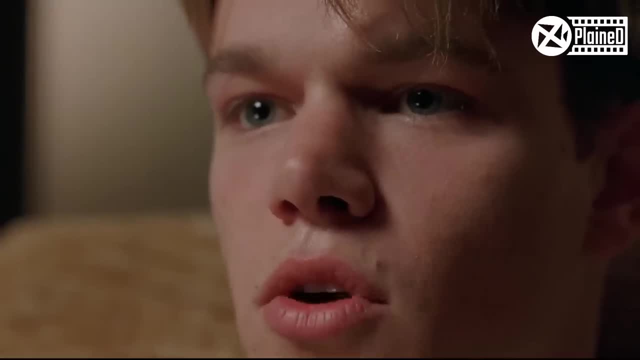 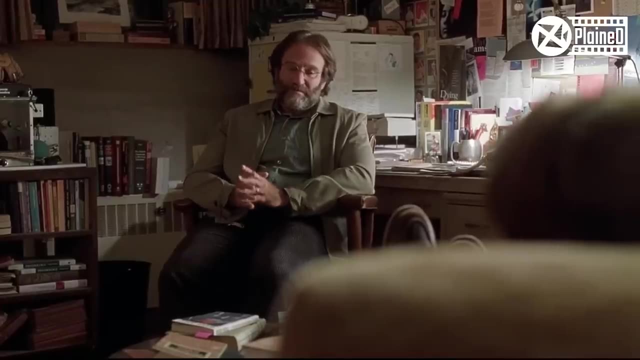 In his therapy session with Sean. he asks who he trusts the most in his life and Will answers Chucky. Sean says that he understands Chucky will give his life for Will, but he will not understand his deep feelings. Sean asks how he plans to earn a living and Will replies that 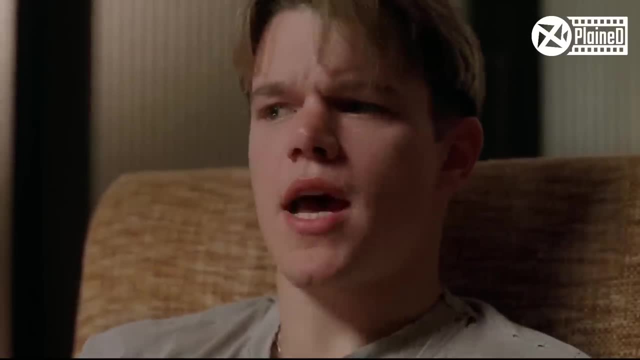 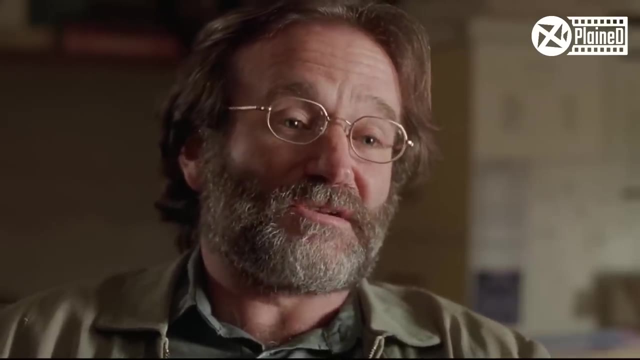 he'll work as a construction worker in Boston for the rest of his life. Sean confronts Will for being scared of living outside of his comfort zone and how it will stop him from living his best life. Sean doesn't force him to take the job that Professor Gerald has planned for him, but he 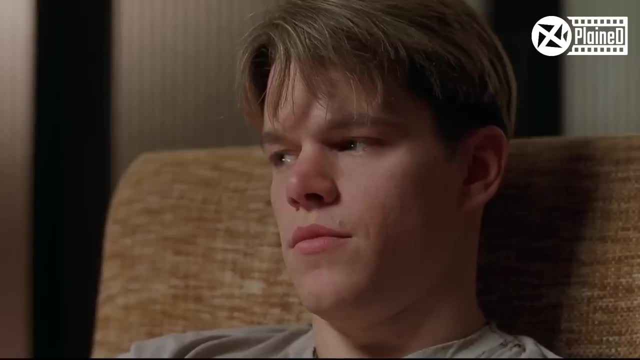 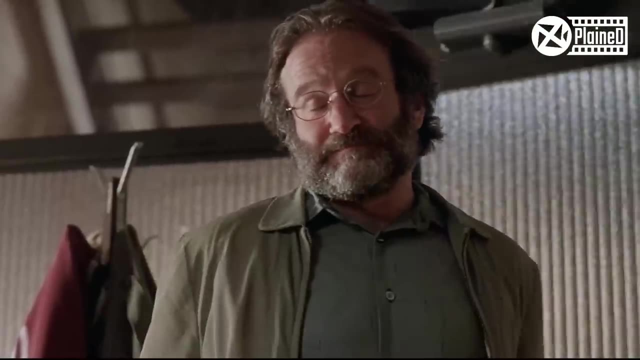 asks Will what he really wants to do in his life? Will replies that he wants to be a shepherd. knowing that Will isn't serious, Sean asks him to leave his office. He says he doesn't want to waste his time if Will plans on not being honest, Will gets angry and starts shouting at Sean. 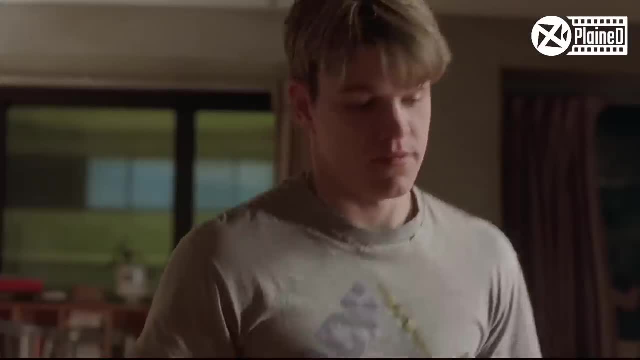 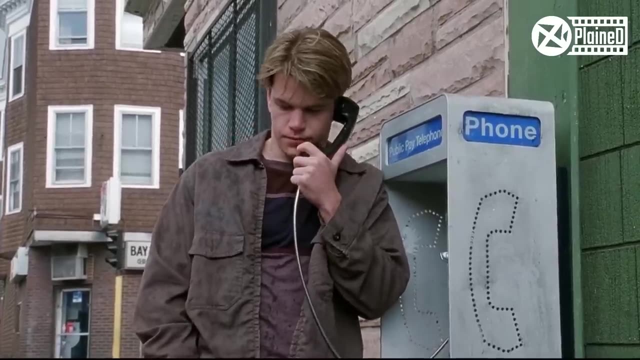 who once again asks him what he wants to do in his life. Will stays silent and doesn't answer. so Sean tells him to leave Before Skyler could leave for California. Will calls her to say goodbye. Skyler, in hope of getting back with Will, tells him that she loves him. Will smiles. 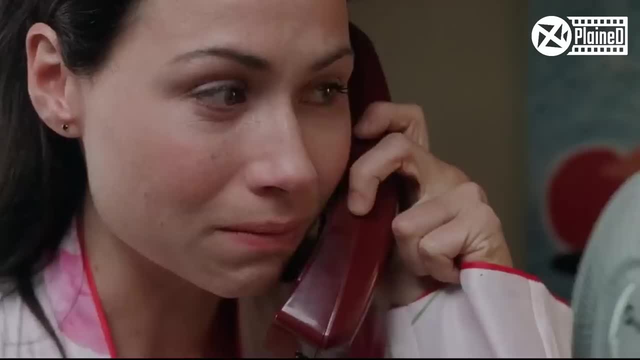 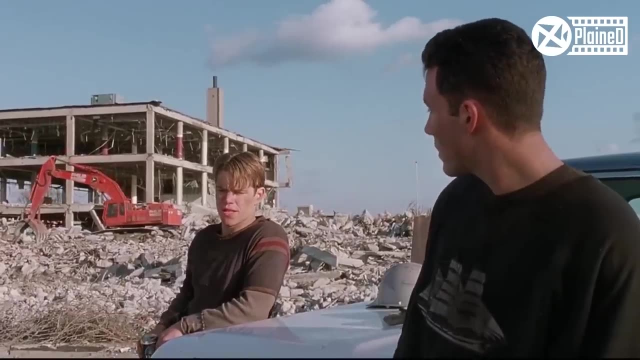 but he has no guts to say it back in fear that he'll only get his heart broken. In his conversation with Chucky, Will tells him that he doesn't plan on getting a job, and he also broke up with Skyler. When asked what he wants to do for the rest of his life, Will answers that he plans. 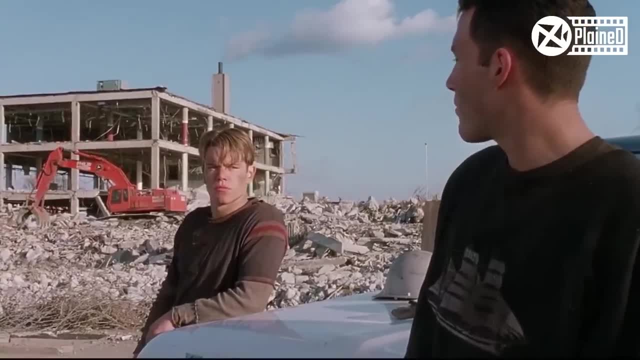 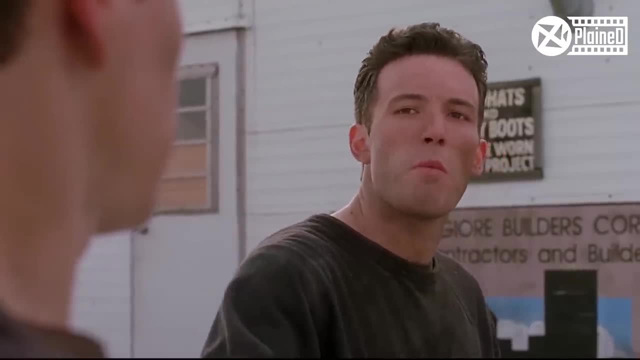 on living in Boston forever, being neighbors with Chucky and working with him on construction. Hearing his answer, Chucky gets honest with him. He tells Will that it pains him to see his friend waste his life when there's more that he can achieve and be happy. Chucky says that he has. 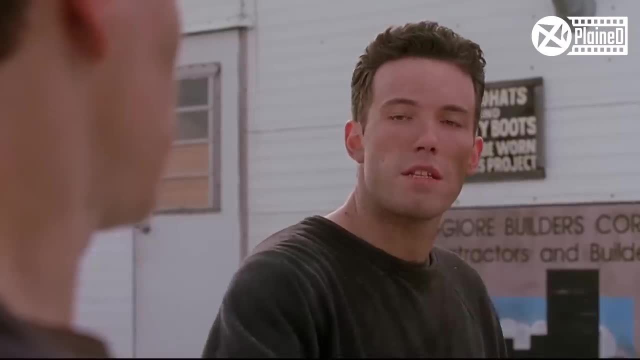 only one wish: Every day, when he comes to pick up Will at his house, he wishes Will wasn't there. Chucky wishes that Will would live with him, but he doesn't. Chucky wishes that Will would live with him, but he doesn't. Chucky wishes that Will would leave his awful life and actually start doing. 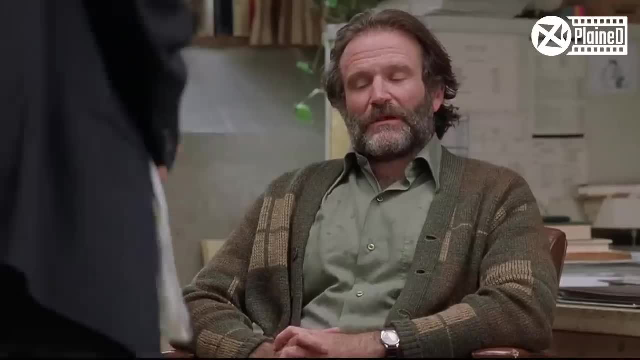 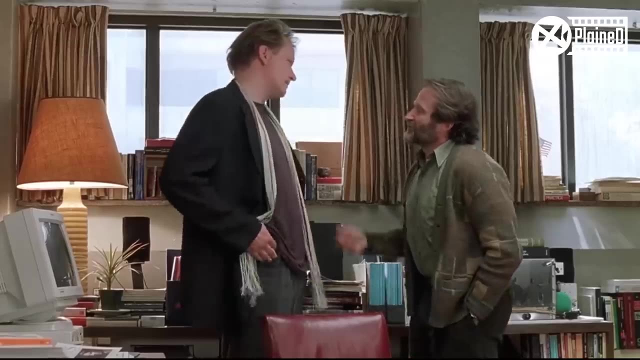 something to make it meaningful. Meanwhile, Professor Gerald is arguing with Sean about how he hasn't been able to persuade Will to get a job and use his intelligence to do something significant in his life. Sean argues that they shouldn't rush into making Will take important. 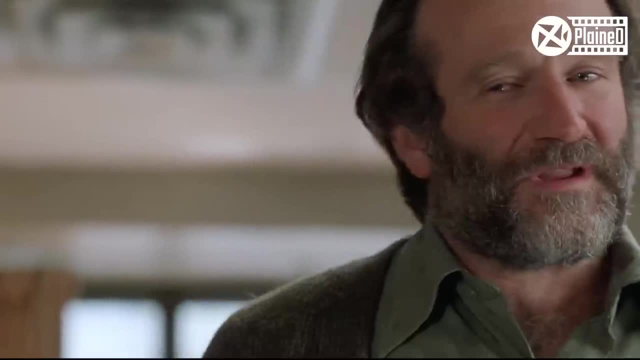 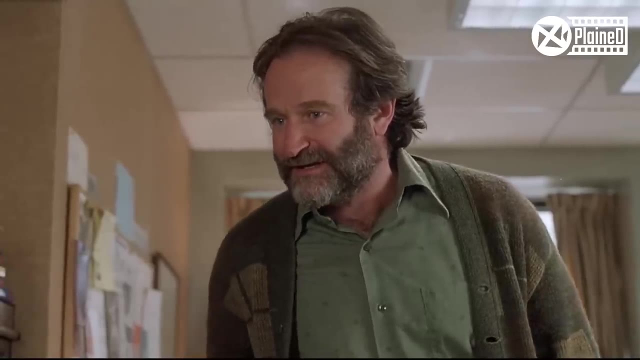 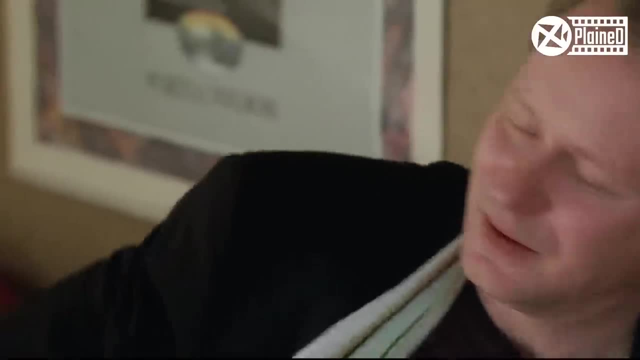 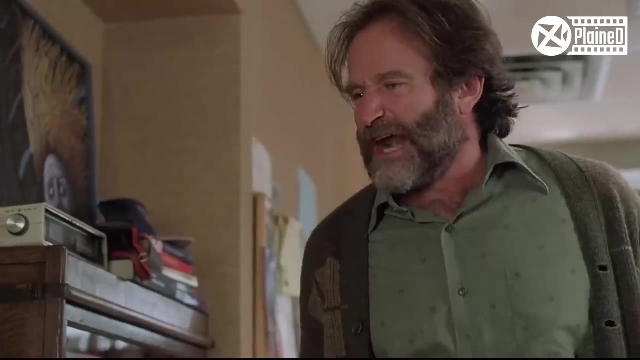 But Professor Gerald doesn't agree with this. He warns Sean to not let Will think that it's okay for him to not make use of his intelligence and spend his life like a failure. The differing views between them ends up into a heated argument, with Professor Gerald calling Sean to be jealous. 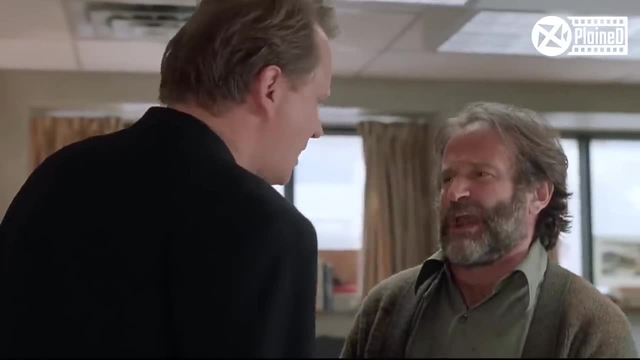 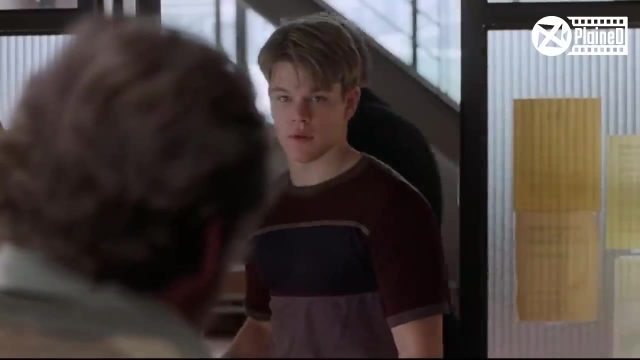 of his success and achievements. Sean tells him that he's not a failure, as he never chose to be like him. Just then Will walks in and hears their conversation. Professor Gerald walks out of the room to let their therapy session begin. Sean has a file which he has pictures of Will's. 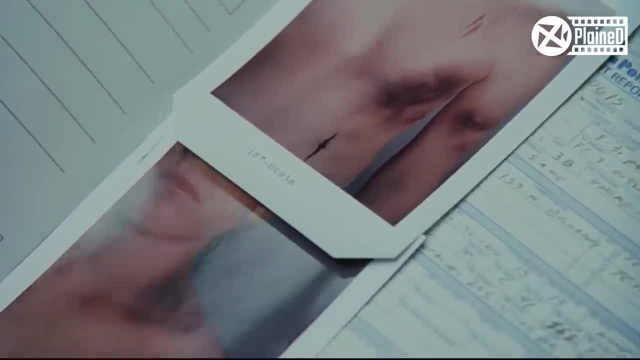 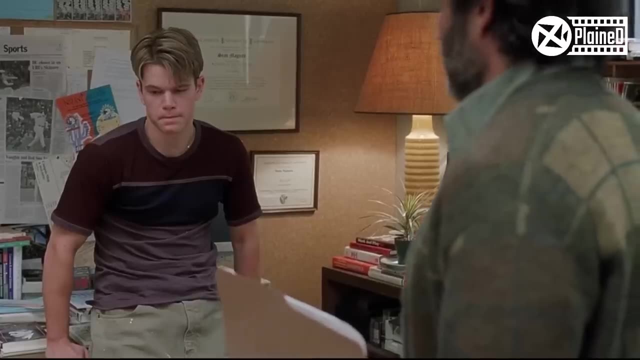 body filled with bruises from the beating he got from his foster father. Will asks if he's seen anything like that before, and Sean reveals that his father was an alcoholic and used to beat him and his mother when he was a child. Hearing Sean's story, Will remembers his foster father. 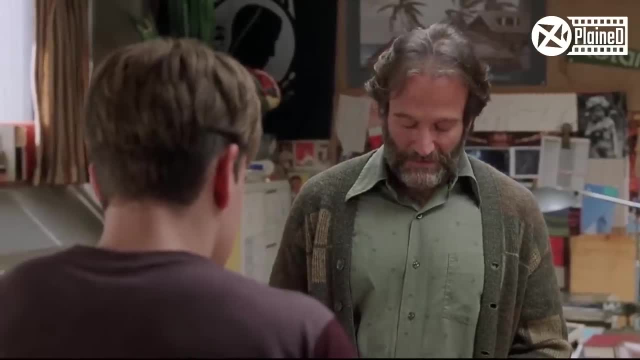 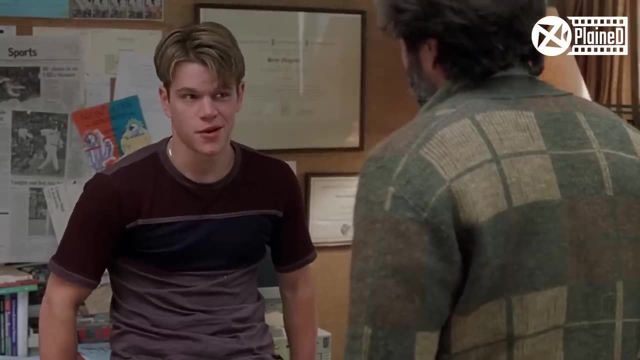 Sean steps in front of Will and tells him that whatever happened to him wasn't his fault. Will nods in approval, but Sean repeats that it wasn't his fault. Will answers that he knows it's not, but Sean keeps on repeating that Will was never at fault for what happened to him. 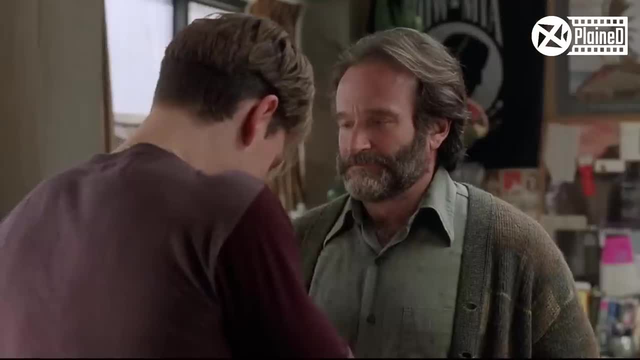 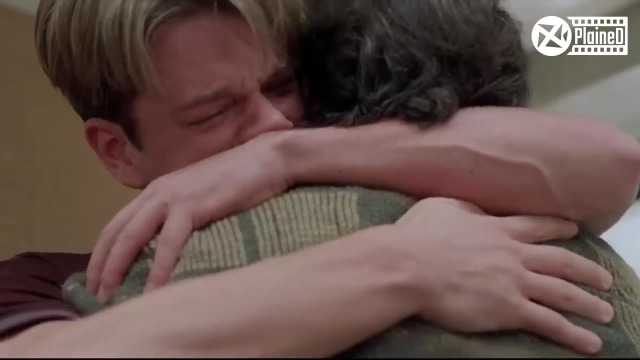 Will says that he's not a failure, as he never chose to be like him. Sean says that he's not a failure at all. Will gets into tears and pushes Sean away. Sean yet again tells him that the abuse he faced as a child was not his fault. Will finally gives in to his emotions and hugs Sean. He cries his. 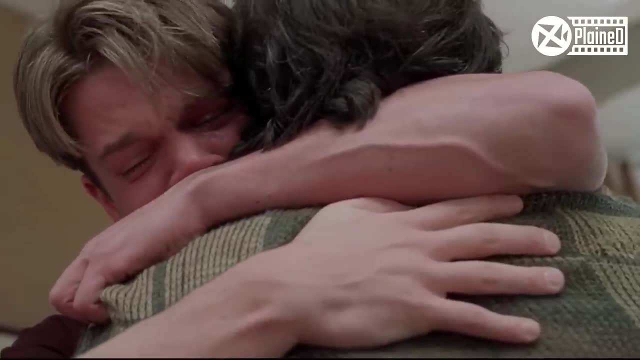 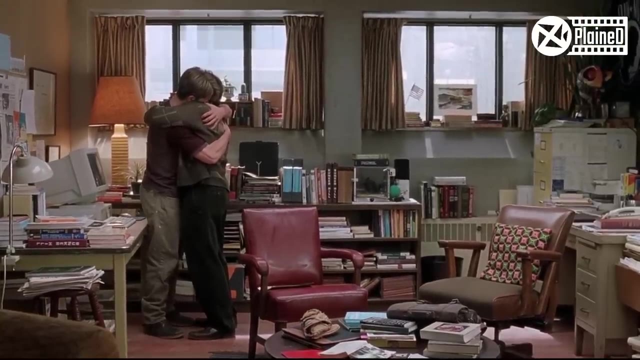 heart out. while holding Sean tightly in his arms, He finally is ready to let go of his past and move on ahead into his life. He tells Sean that he's going to take one of those jobs that Professor Gerald has set him up for. With this, his final therapy session with Sean is over. 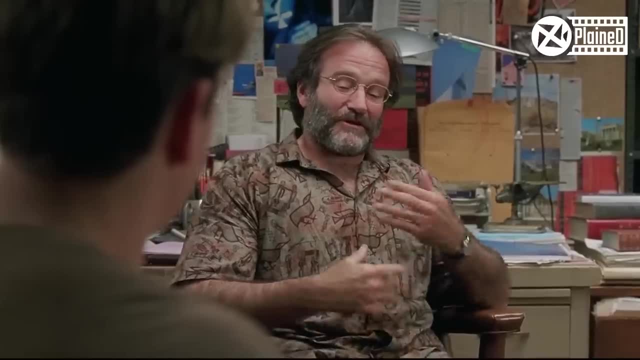 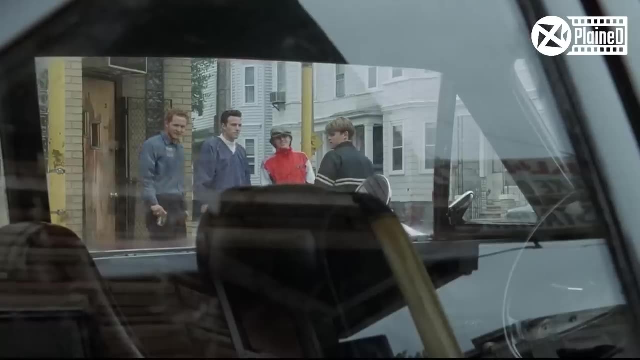 Will asks if he can stay in touch with him and Sean replies that he's always there for him and tells him to do what his heart wants. Will hugs Sean before bidding a final goodbye. As a gift for his 21st birthday, Chucky, Billy and Morgan give him a car. The car isn't brand new, but Will is happy with the gift. 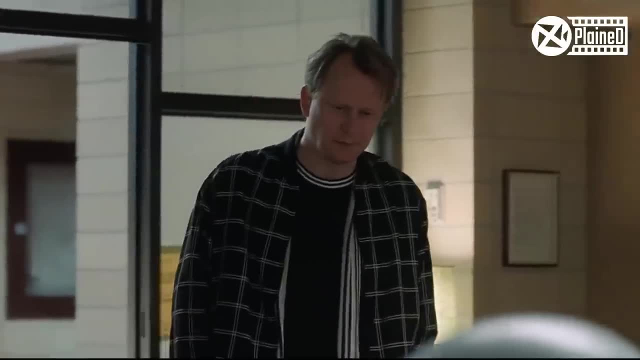 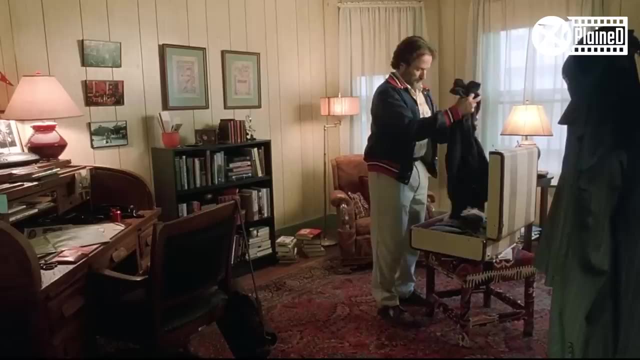 as it's from his best friends. Meanwhile, Professor Gerald goes to Sean and apologizes for what he said to him. The two friends reconcile and Sean tells him that he's going on a world tour. While Sean is packing his luggage, Will drives up to his house and watches him getting ready for his trip. 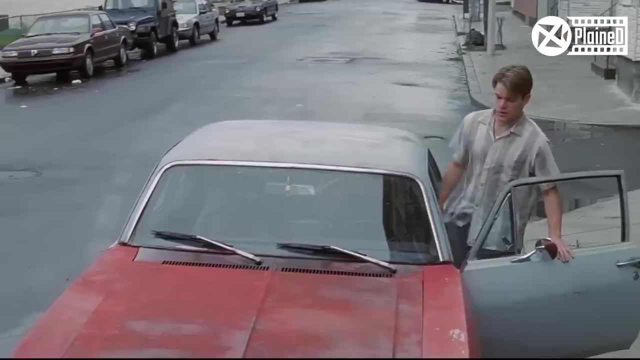 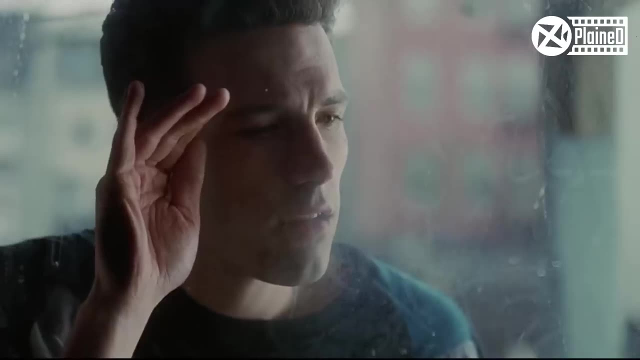 Will walks to the front door and places a letter in Sean's mailbox before driving out. In the meantime, Chucky goes to pick up Will at his house. He knocks on the door but gets no answer. He peeks in through the windows and sees that Will isn't home. Chucky smiles as he realizes that Will has 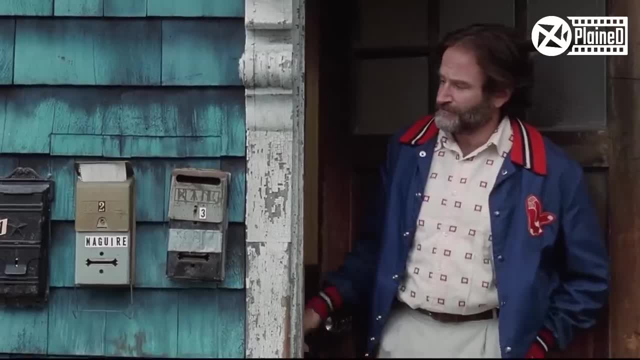 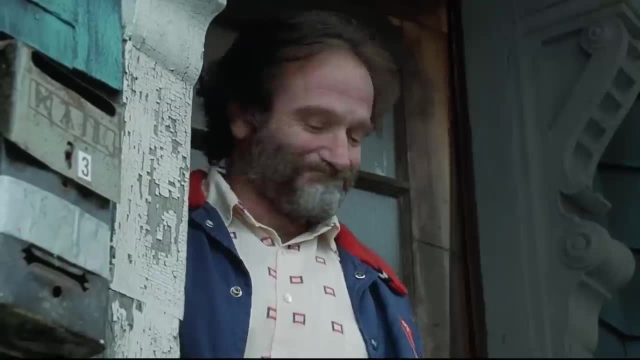 finally decided on what he wants to do with his life. Sean also gets the letter left by Will. In the letter, Will writes that he's not taking the job and he's going to California to meet Skyler. Sean smiles and goes back to his house And the movie ends. 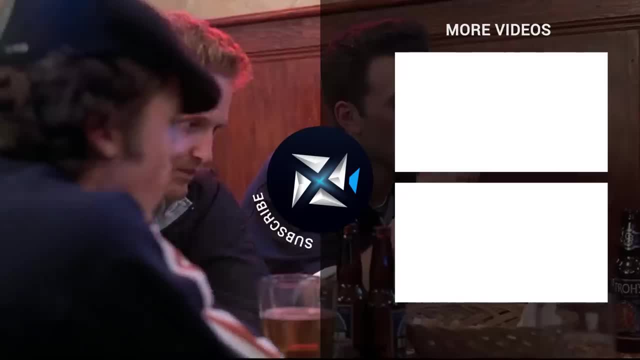 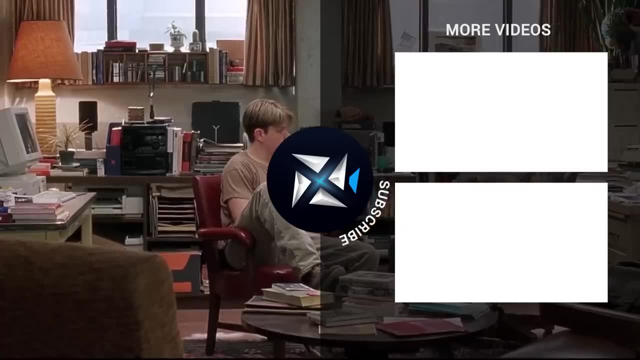 As we see, Will on his way to get back with Skyler. Thanks so much for watching. Tell us your thoughts on the movie down below in the comment section. If you enjoyed the video, please leave a like and do watch some of our other videos. 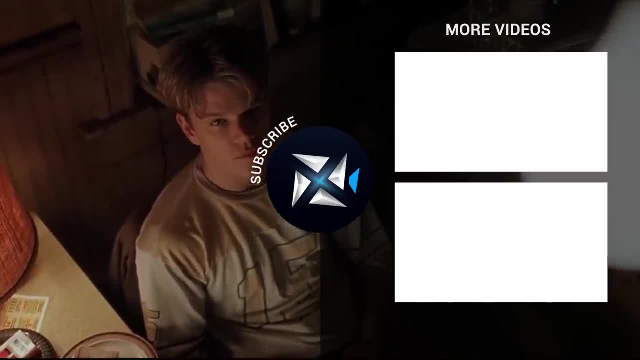 as well, And before you leave, make sure to subscribe to the channel for more movie recaps.